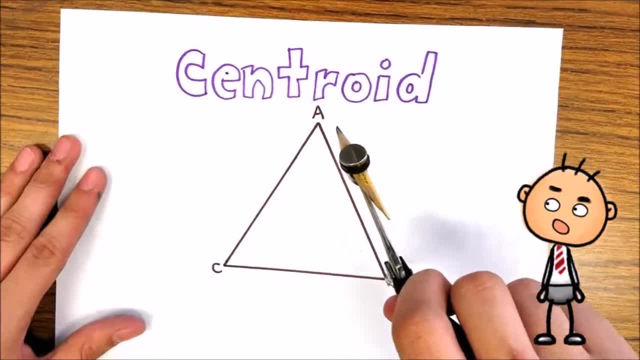 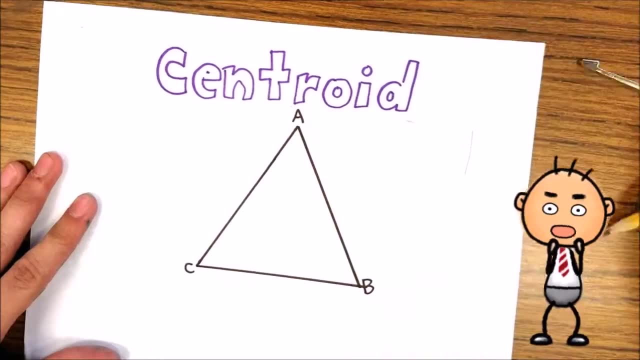 Extend the protractor to the length of the side you are working with Now make an arc on the top and bottom of the side. Next switch the length to the other point of the side and make an intersecting arc on the top and the bottom. 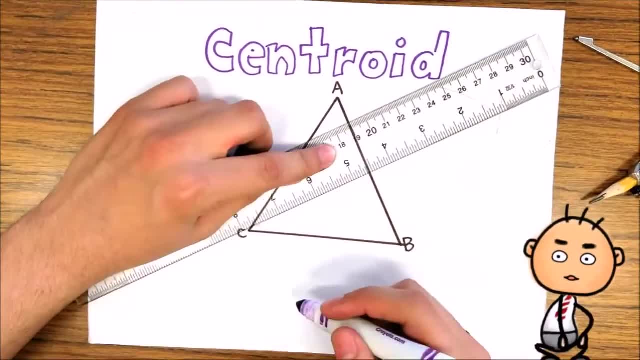 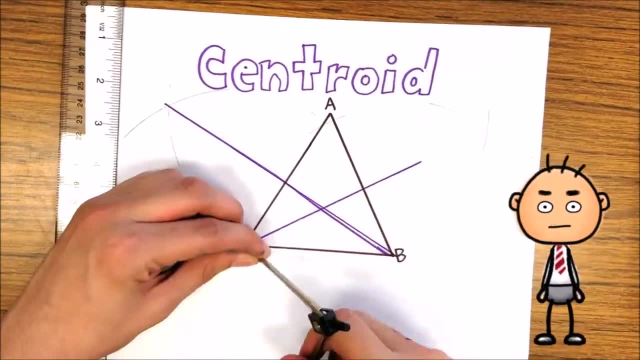 Finally, use a straight edge and draw a line from where the two arcs meet to the opposite vertex. Repeat the same steps for the other two segments. When finished, you should have three lines meeting in one place, and that is the centroid, The incenter. 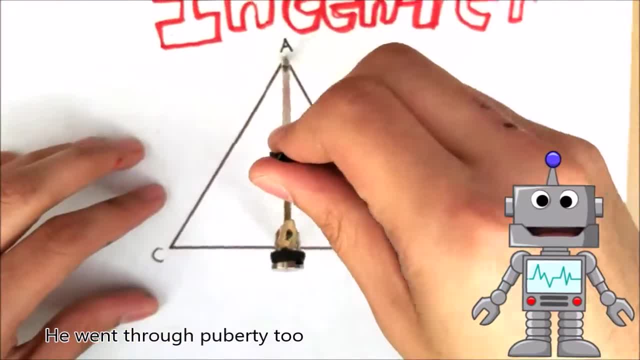 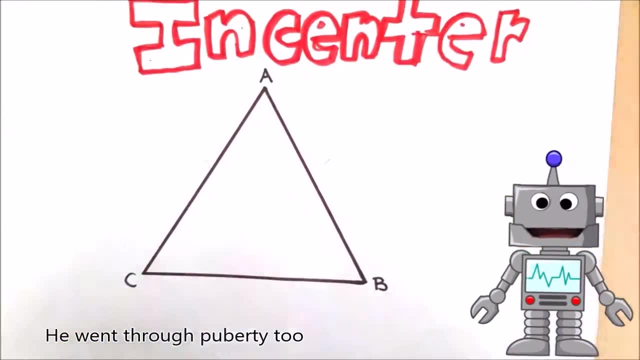 First choose one of the corner from the three vertices to work with. In this video I will be using vertex A. Using the leg of a compass, you mark the chosen vertices and adjust the hinge to to extend the pencil further to mark the two side adjacent to angle A with equal length. 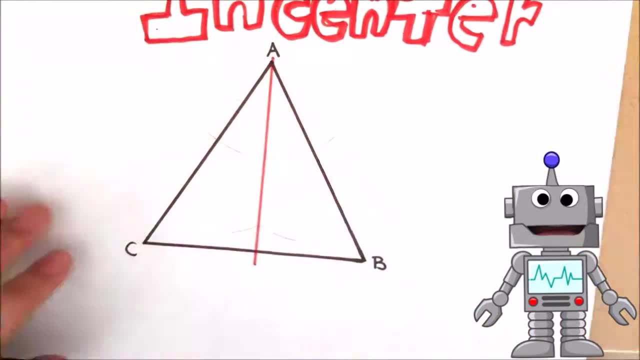 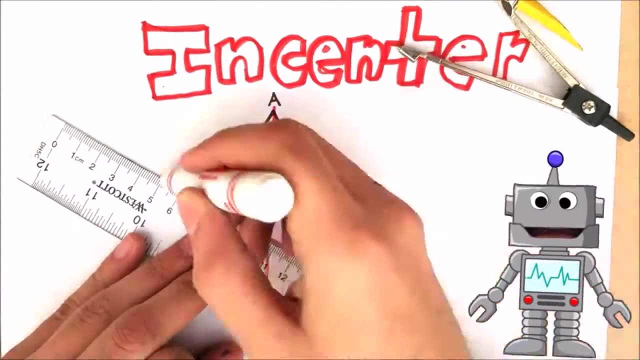 Remove the compass and place the leg on the marked side and create an arch. Repeat this on the other marked side and create the same arch to intersect the previous arch, Using a straight edge, draw a line from angle A to the intersection and extend it. 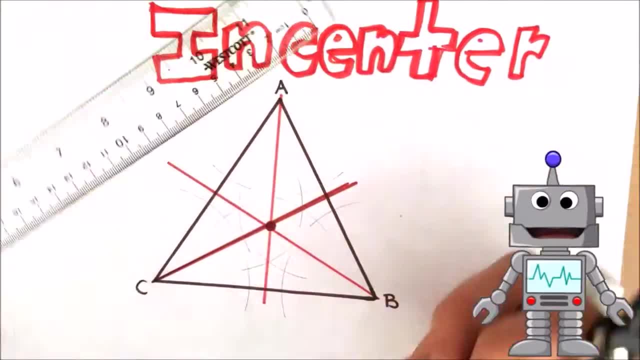 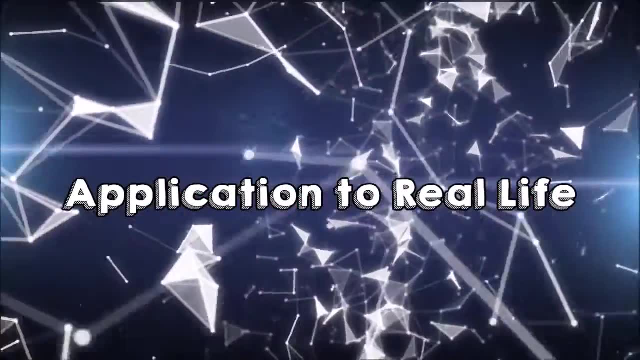 Apply these steps to the other two angles to find the incenter. After you find the incenter, you can draw a circle using the point inside the triangle. The circle will touch all three sides of the triangle. The centers of the triangles can be used several different ways in real life. 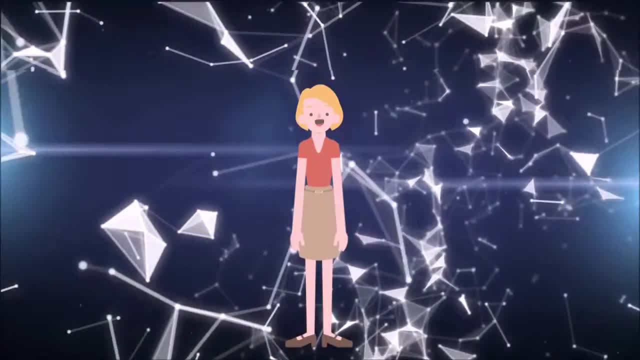 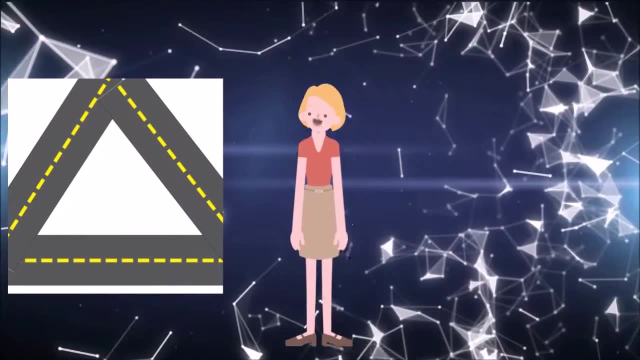 For example, the incenter can allow us to place an object equidistant from the sides of a triangle, like a triangular road. Say, a park has a triangle road and the builders want to add a fountain equally distant from each road. They would find the incenter of the road to do so. 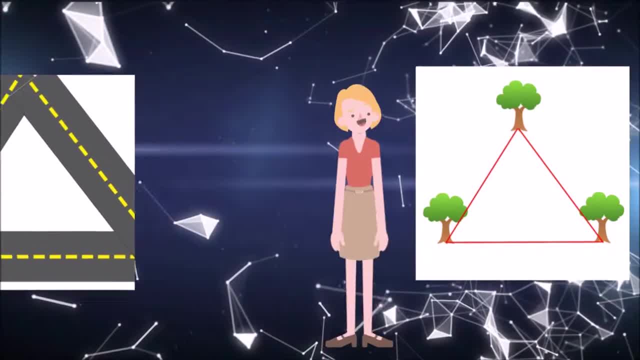 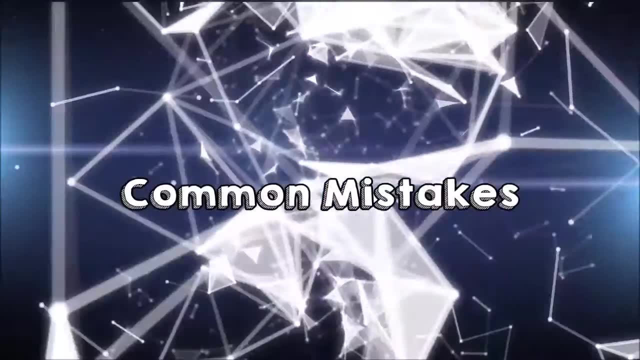 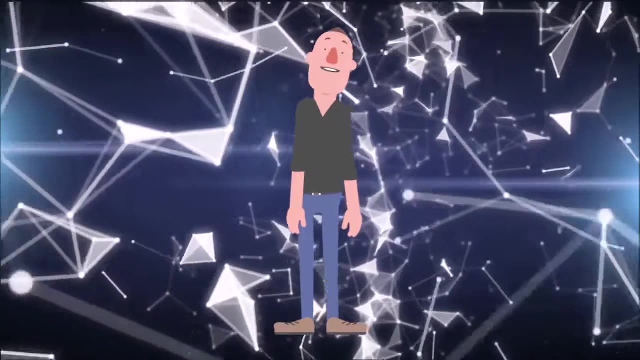 If there were three trees in triangle shape in a park and the builders wanted to place a bench equidistant from each tree, they find the circumcenter of the three trees. Often, students get confused with the four different types of triangle centers, which causes them to confuse the steps. 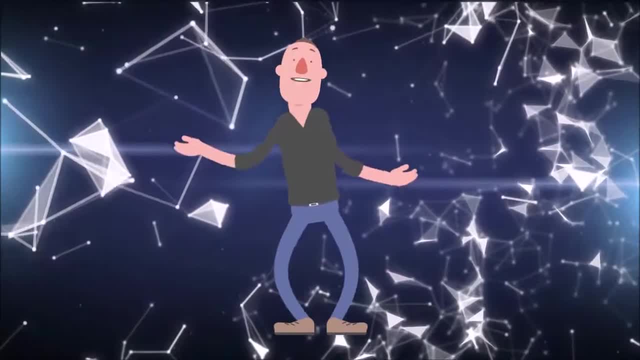 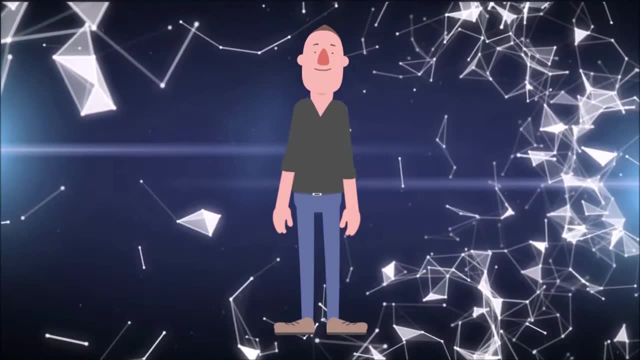 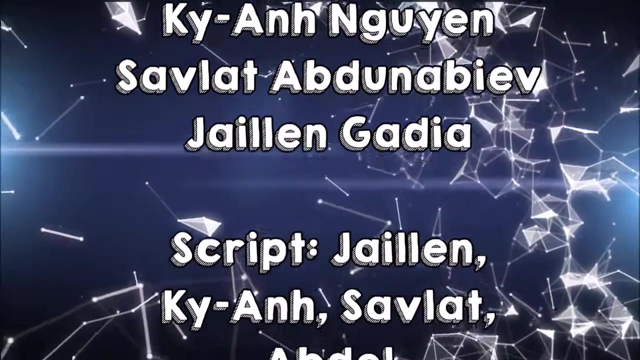 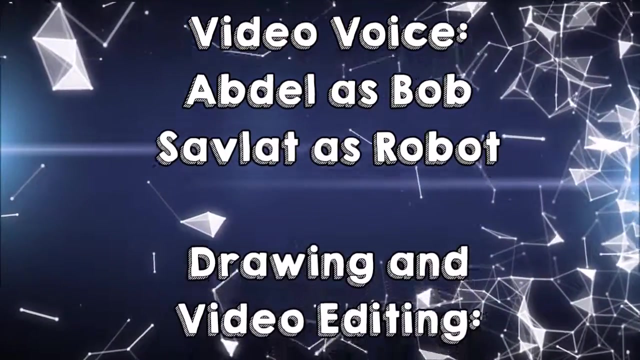 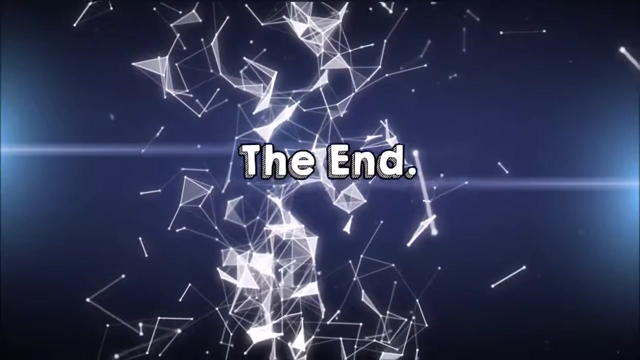 Also a common mistake is when a student's protractor slips on the paper or moves without them realizing. That can cause them to not get intersecting lines for the triangle centers, since the marking will be off. For example, they might think that a blank space has nothing to do with a figure on a board, so a rectangle would not mean that it has a passenger or thingija.